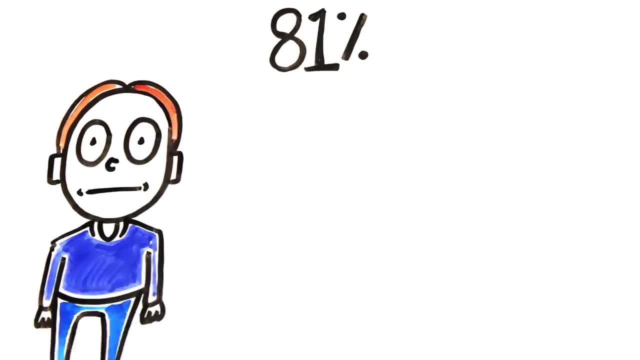 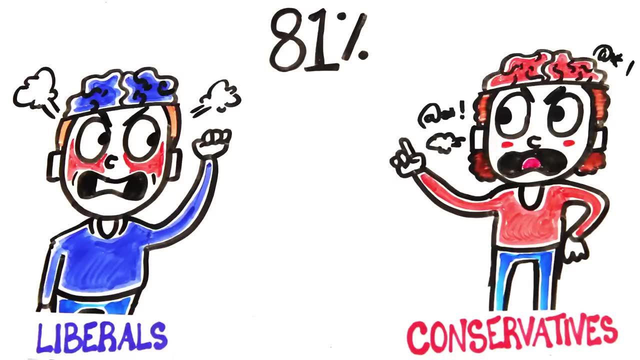 The world feels pretty divided. Currently, 81% of both liberals and conservatives have unfavorable views towards those on the other side. But is there actually a fundamental biological difference between liberals and conservatives? On the surface, we can see some funny differences, like conservatives like meat and potatoes. 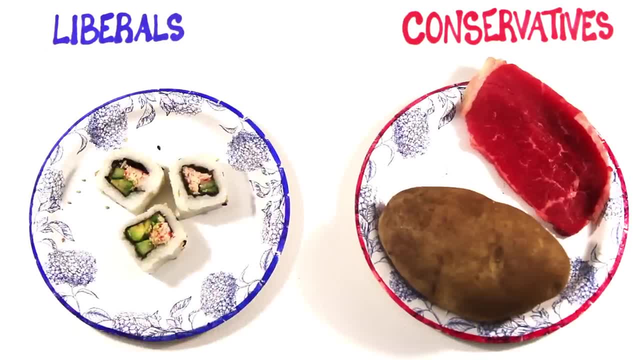 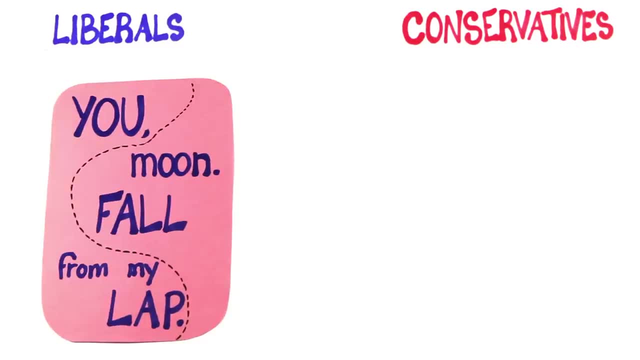 more, while liberals tend to like trying food from other cultures more. In general, conservatives prefer purebred dogs while liberals prefer mixed breeds. And liberals are okay with free verse poetry, while conservatives prefer it to rhyme. But as we study more, we realize. 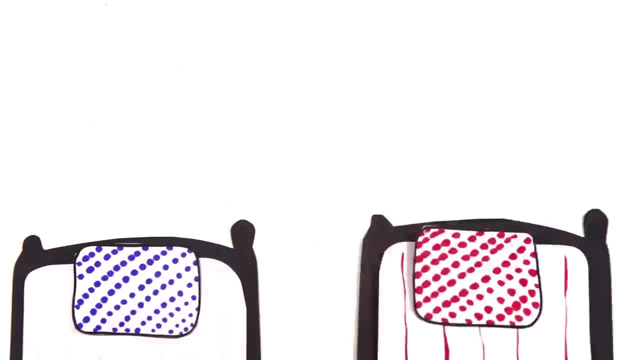 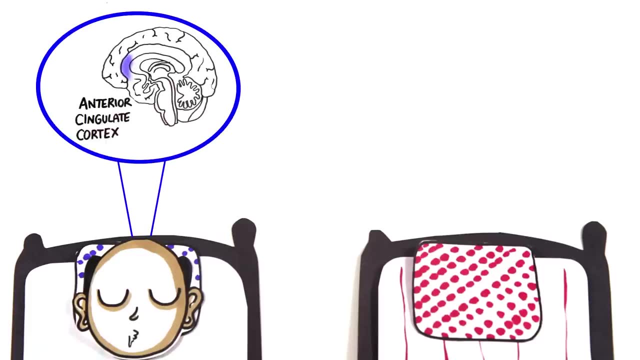 that the differences are much deeper When put through MRI brain scans. it turns out that liberals are more likely to have a larger anterior cingulate cortex, which is associated with understanding and monitoring conflict, while conservatives have a larger right amygdala, which helps process fear and 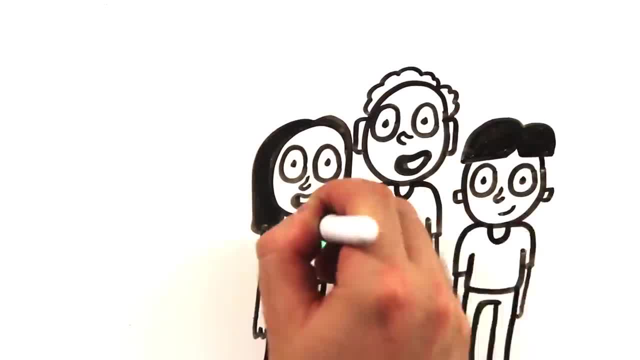 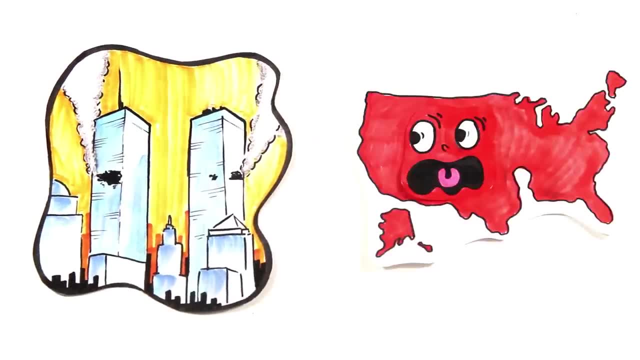 anxiety, And that makes sense, given the years of research that have shown people tend to become more conservative when they feel threatened or afraid. After 9-11,, for example, the US became politically more conservative, with studies showing increased support for issues like national security and military spending. 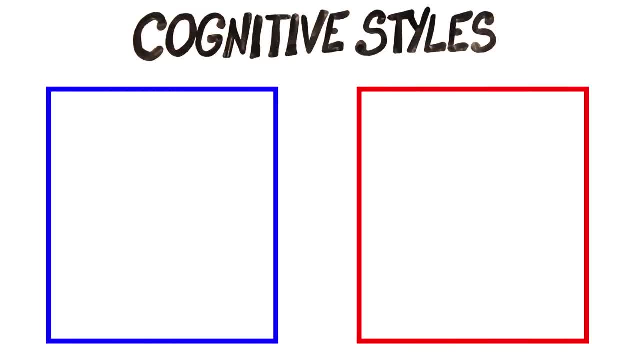 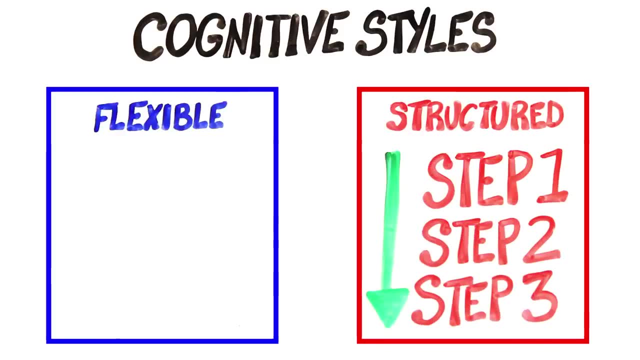 But studies have also found that conservatives and liberals employ different cognitive styles. Conservatives excel when it comes to more structured and organized problems or questions, whereas liberals tend to be more flexible and less likely to commit errors with questions involving conflicting information and requiring fast reaction times. One study looking at 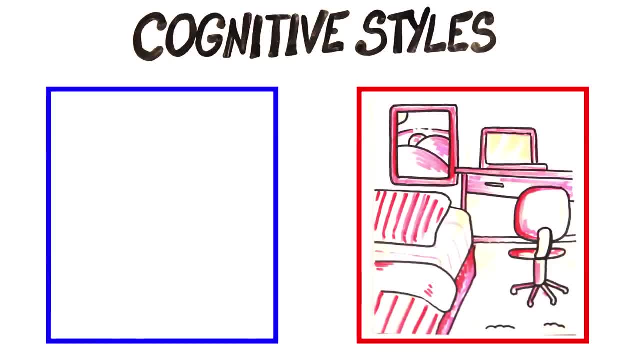 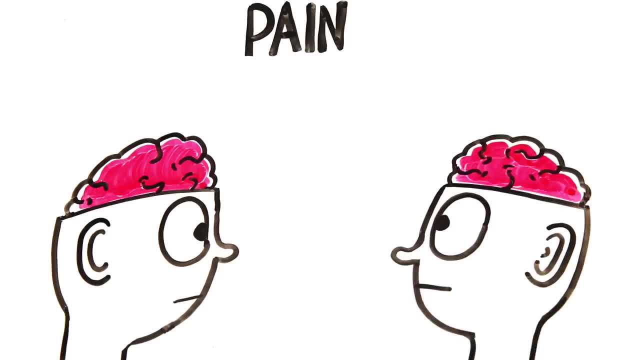 dorm rooms, even found that, on average, conservative students' rooms were less messy than liberals'. But they also experience pain in different ways, so much so that one study was able to predict who was liberal or conservative just by viewing brain scans of them looking at. 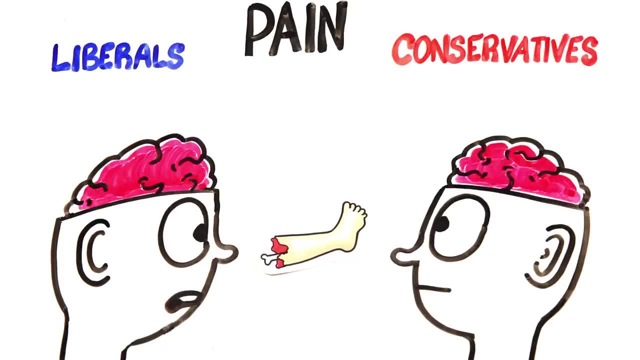 graphic photos containing mutilations. In this instance, liberal brains were more active in the S2 or somatosensory 2 region, which is normally activated when you're in pain, but also when you see someone else suffering. It's essentially scientific evidence for the bleeding heart liberal stereotype, which doesn't 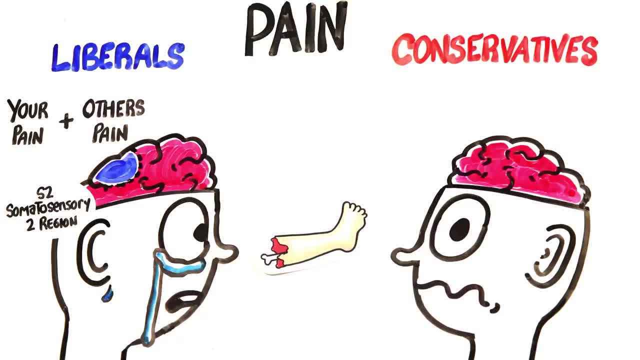 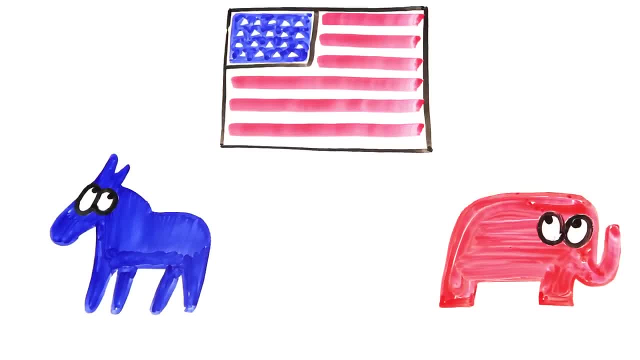 mean conservatives are uncaring, But that their minds are more sensitive when they're in pain than they are when they're suffering. Republicans just respond to graphic images differently In America. this can explain how Democrats and Republicans perceive the world in fundamentally different ways.